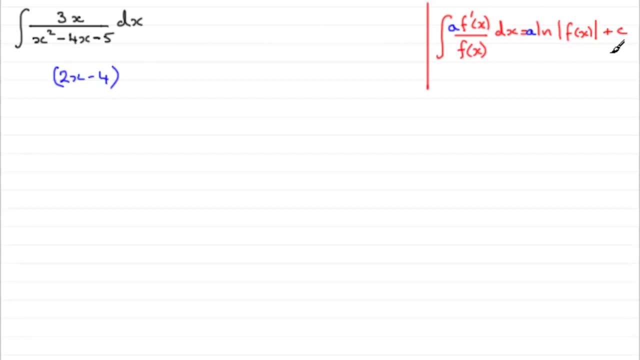 So it's not one of these types, well, certainly doesn't appear to be at the moment anyway. So how do we do this? Well, the next thing we look at is: does the denominator factorize? And it does. So let's factorize it and we'll see where we go from there. So let's factorize f into. 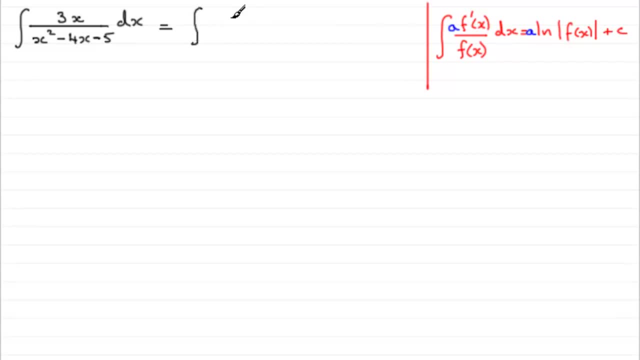 f? dash of x plus b. Then we'll get f? dash of x plus b And we'll see where we go from. we go from there, so we'll have the 3x there, and this quadratic expression then splits up into two brackets. there'll be an x minus 5 and an x plus 1, and that will have dx on the end. 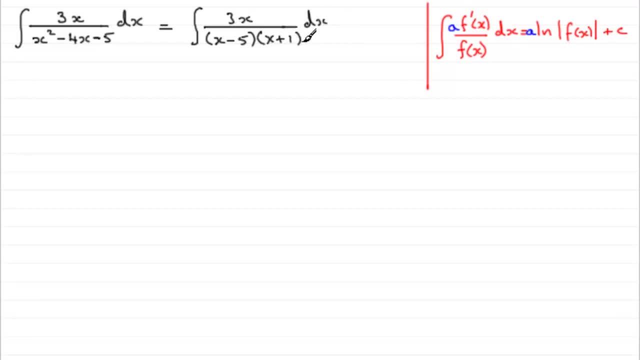 okay, so we've now factorized the denominator. so what well? the point is that when you get something like this and you can factorize the denominator, we can split this up into partial fractions. so hopefully your partial fractions are okay. if not, just look on my tutorials for. 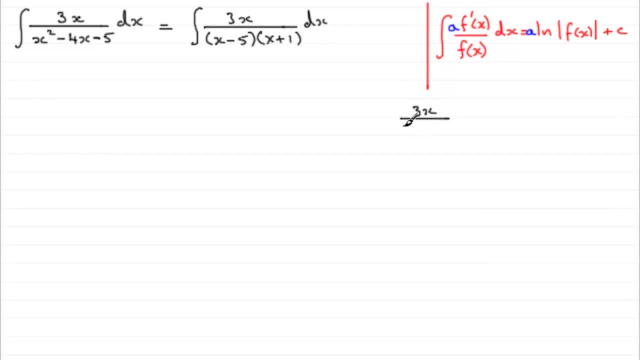 working with partial fractions and a, And we'll do it here anyway: 3x over x minus 5, x plus 1.. Now these are linear factors: the x minus 5 and x plus 1.. And so this is identical to a constant. let's call it a over the first linear factor, x minus 5, plus another constant, b over the other linear factor, x plus 1.. 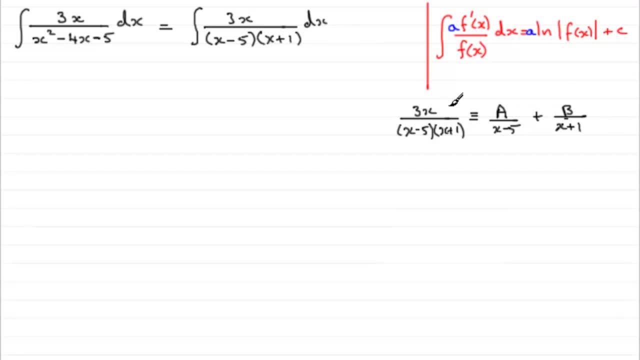 And there's various methods of solving these. What I tend to do is multiply both sides now by x minus 5 and x plus 1.. And so that's going to give me 3x is identical to a multiplied by x plus 1, and then b multiplied by x minus 5.. 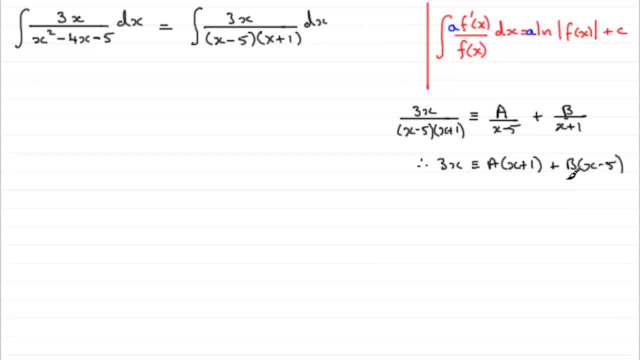 As I say, if you're not sure of this, just go on my website. look under partial fractions in the tutorial index. Now We need to work out a and b, so what we can do is select x to be minus 1.. 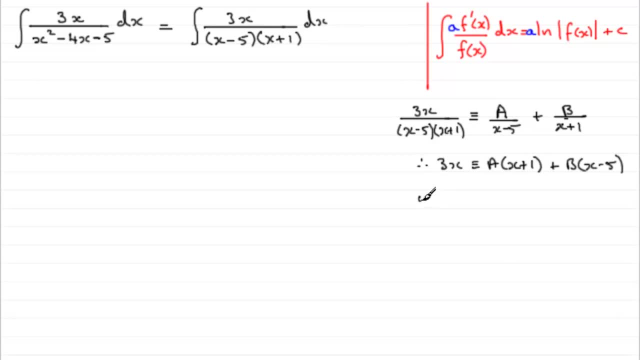 It'll make this bracket 0 and take out this term. So when x equals minus 1, we have 3 times minus 1, which is going to be minus 3.. And that's going to equal, well, minus 1 minus 5 here is minus 6, so it's minus 6b. 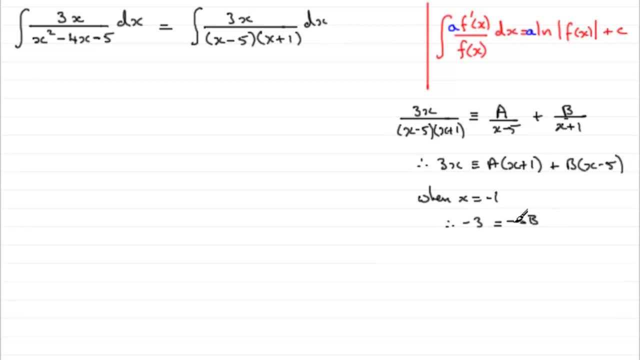 And if we divide both sides by minus 6, b is going to be Minus 3 over minus 6, which is a half. So b equals one half, And to get a I make this bracket 0, so I let x be 5.. 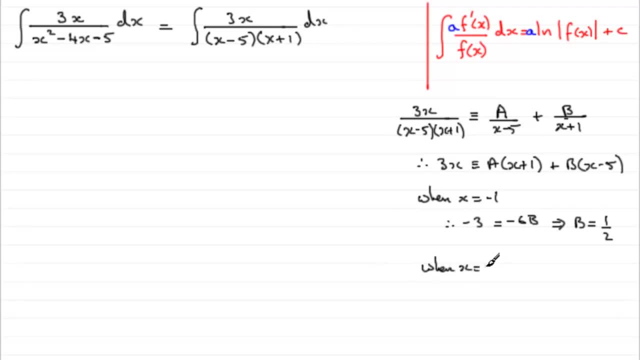 So when x is 5, OK, we have 3 times 5 there, 15.. In other words, we therefore have 15 equals. put 5 in here. 5 and 1 is 6, 6a. 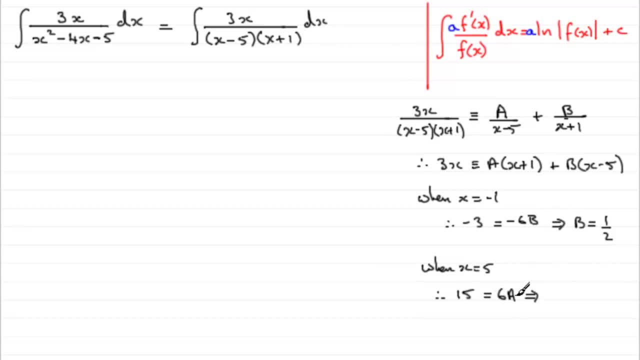 So it follows from here: If we divide both sides by 6,, that a equals 15 over 6.. And we could divide both top and bottom by 3, and that will give us 5 over 2.. So what this is telling us, then, is that this value here 3x over x minus 5,. 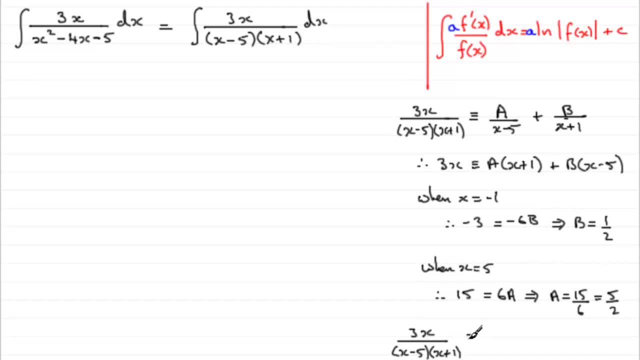 multiplied by x plus 1, is identical to a over x minus 5.. So a was 5 over 2, so we're going to write that as 5 over and pull the 2 down here, and that will be x minus 5.. 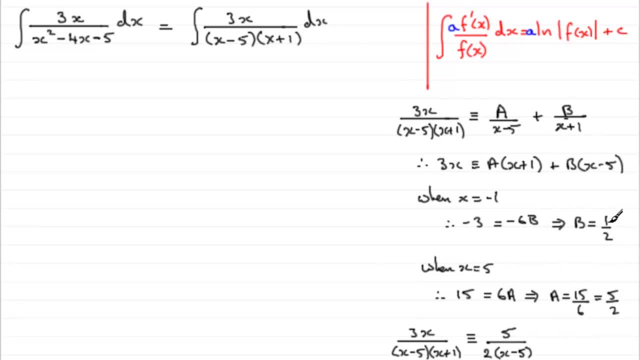 And then we've got plus b over x plus 1.. b was a half, so we've got plus 1 over 2. lots of x plus 1.. So we need to do this kind of thing. Let's just border that off there. 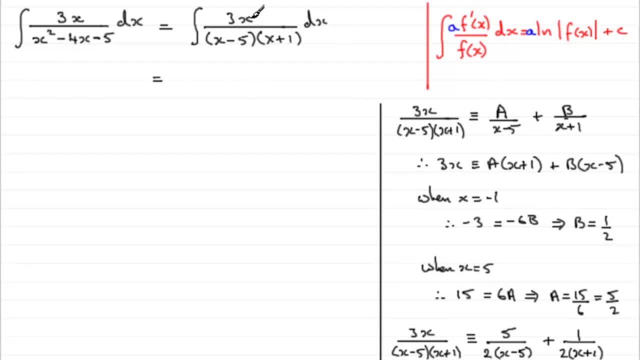 OK, so let's carry on with this. So we've got this integral. now We've split this into partial fractions, So we can rewrite this as this: OK, Now what I'm going to do is because we've got 5 and the 2, they're constants. 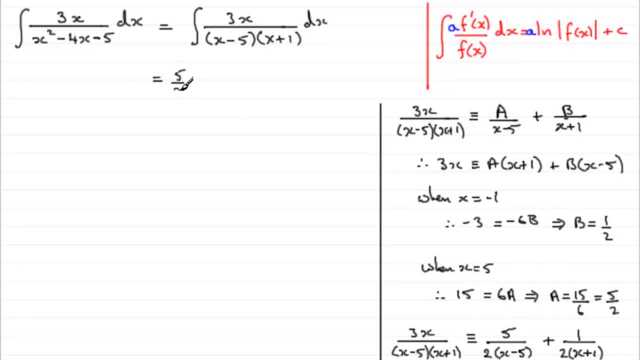 I'm going to pull them out the front of the integral. So we've got 5 over 2, and then we've got the integral of 1 over just the x minus 5.. So we've got that one. we'll put a dx there, OK. 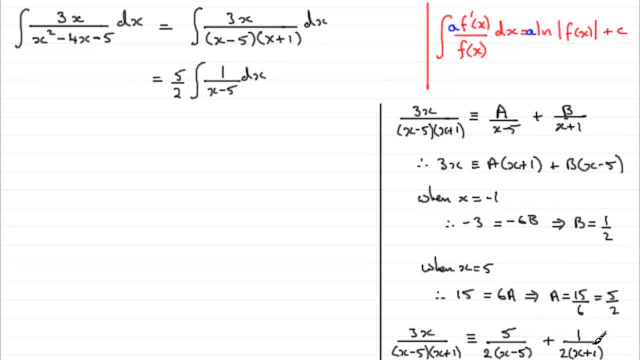 And then we've got the integral of 1 over just the x minus 5.. And then we're going to integrate this one And similarly we're going to have one half out the front of the integral A half. then you have the integral of 1 over just the x plus 1.. 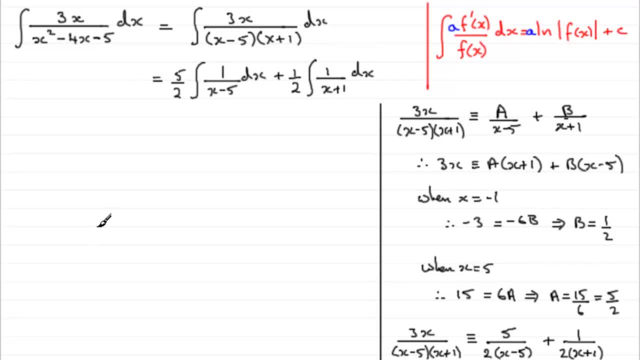 And again, not forgetting the dx there. OK, so how do we go about integrating this? Well, it's a fraction And, as I said earlier, any time I have a fraction, I would always check out this rule. If I differentiate the bottom, I get just 1.. 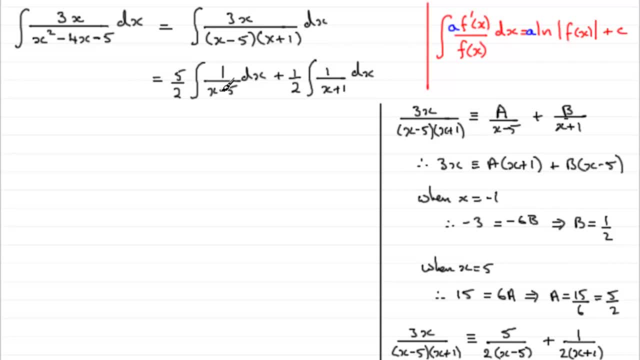 And that's what I've got on the top here. So this is a natural log type, the natural log of the mod of x minus 5.. So what we have then is 5 over 2, then multiplied by the natural log of the mod of x minus 5.. 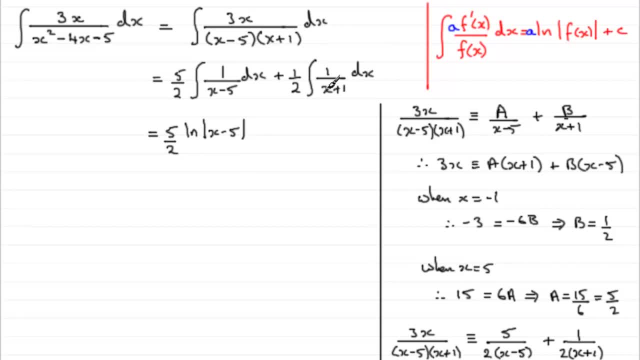 And similarly for this one. can you see that when you differentiate x plus 1, you get 1, which is the value on the top. So this is going to be plus a half, multiplied by the natural log of the mod of x plus 1.. 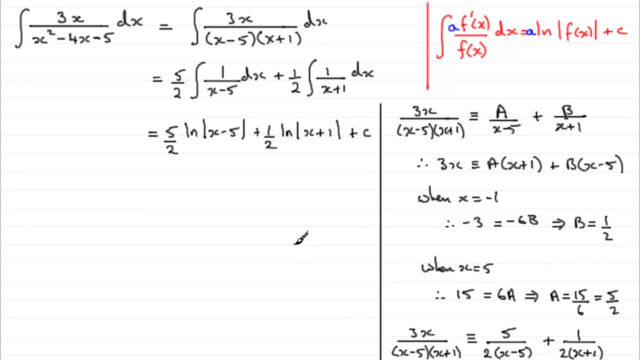 And then we shouldn't forget the constant of integration plus c. Now you could leave it like this, but quite often we can simplify these further by using the rules of logs. What we need to do, or what we can do, is we can see that half is a common factor here. 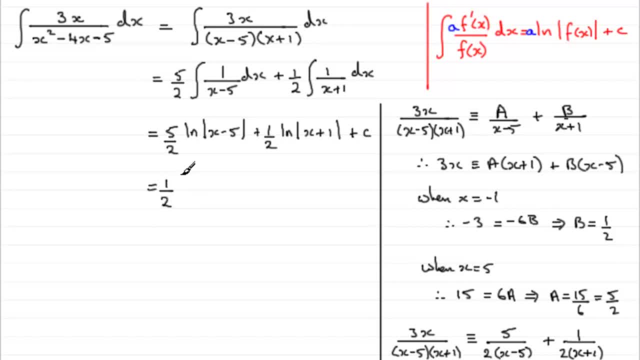 So we could pull out half in this particular example and then write 5 multiplied by the natural log of x minus 5, and then plus the natural log of x plus 1, and then close the bracket off plus c. Can you remember that if you've got the natural log of something plus the natural log of another value, 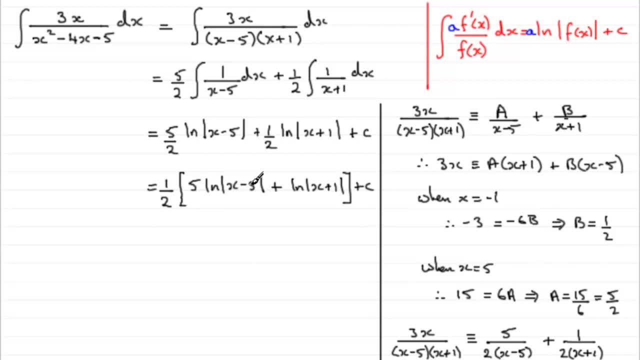 it's the same as doing the log of one value multiplied by the other, but you mustn't have a number in the front for that to work. But when you've got a number in the front we can take this up as a power.